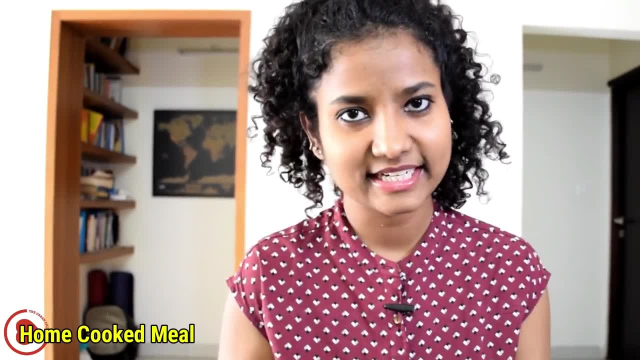 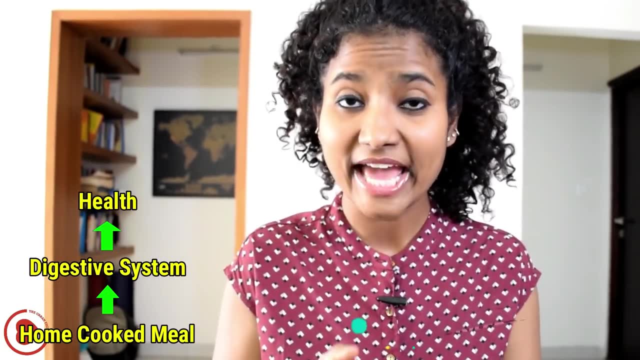 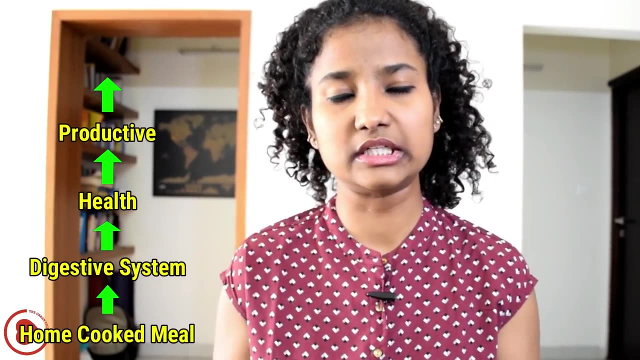 one basic thing: A home-cooked meal takes care of your digestive system. A good digestive system takes care of your health. Good health makes you active, That makes you productive, And productivity leads to a great career, good friends, more money, And that is how you become. 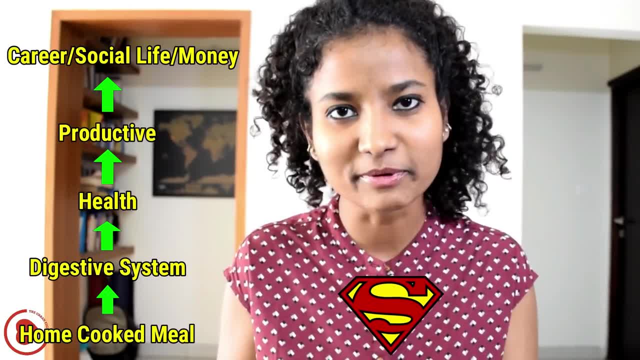 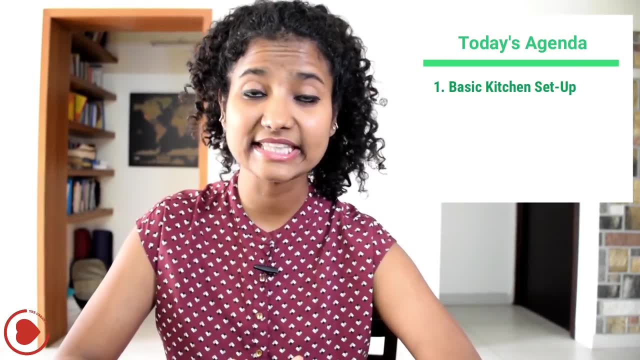 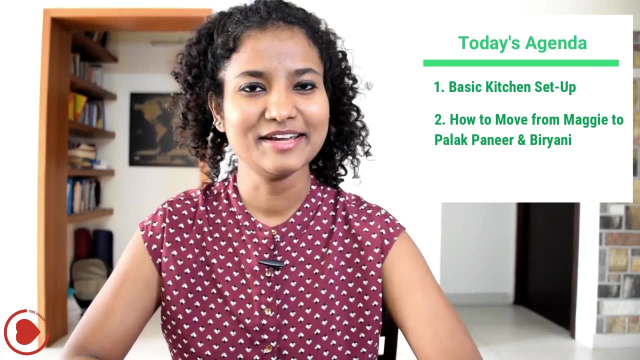 the hero of your story. So if you want to become a superhero, you need to learn how to cook, Hence proved. So today I'm going to tell you what all you need in the kitchen to start cooking, How I transitioned from maggi to palak, paneer and biryani, But, most importantly, in the end. 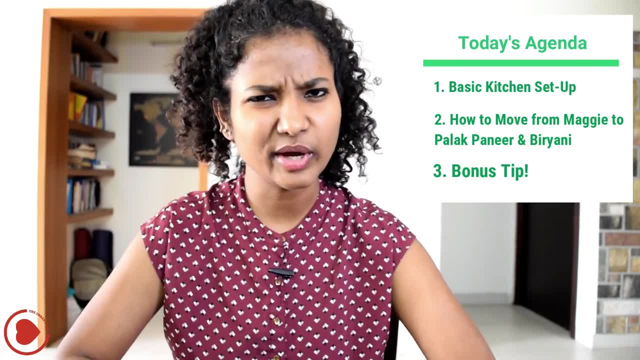 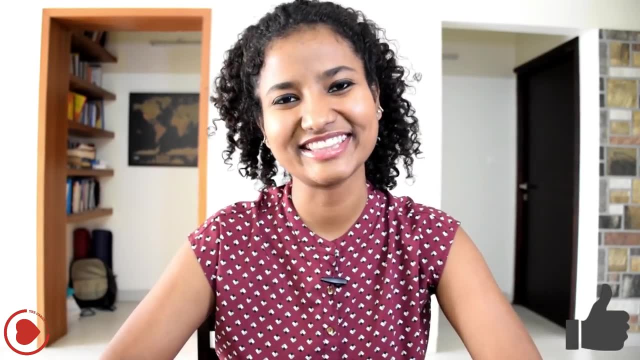 I'll give you a bonus tip So that, even if you hate cooking, you'll start enjoying it. But before that, if you like me, or if you like what I'm saying, hit that big fat like button. Let's begin. 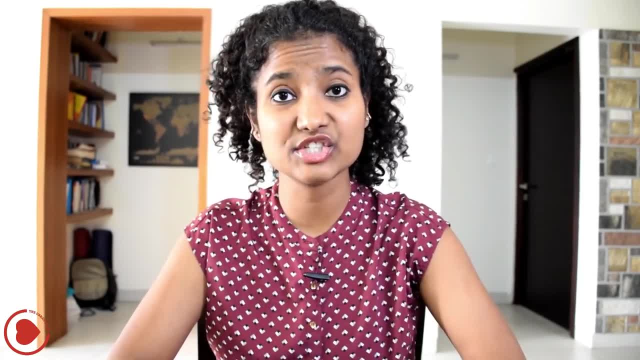 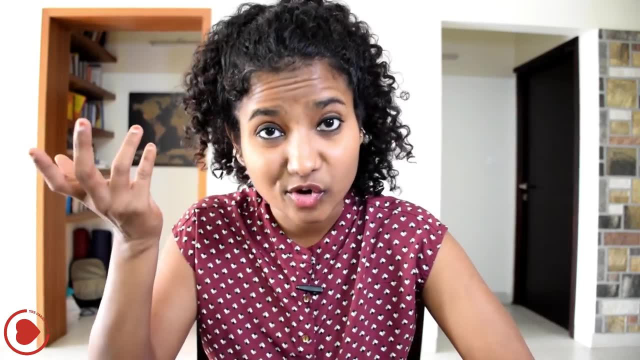 So today I'm going to tell you how you can learn cooking, like I did, in just five days. Let's start with day one. Before you can even think of cooking, you first need to organize your kitchen. So take out your notes, because I'm going to tell you what all you need to shop for. 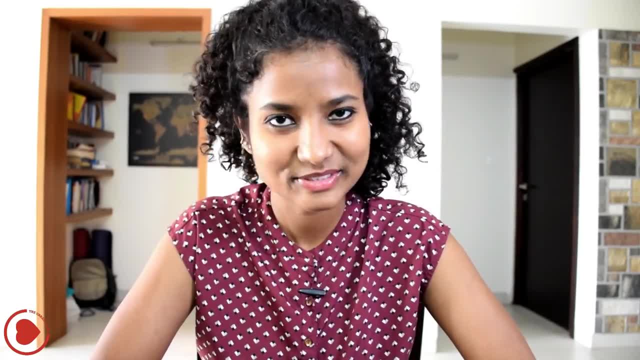 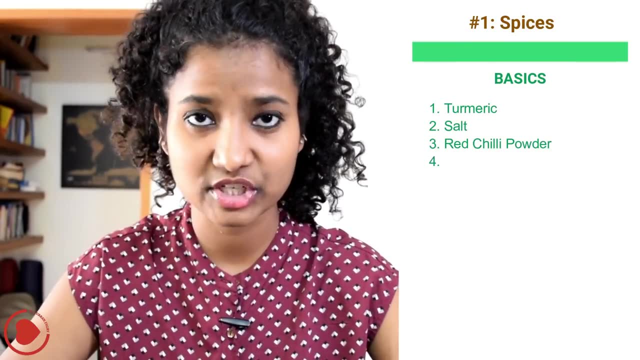 from the supermarket or your local sabji mandi. I've divided the kitchen supplies into six categories. First is spices. Let's start with the basics: Turmeric salt, laal mirch, jeera rai, coriander powder, jeera powder and garam masala powder. 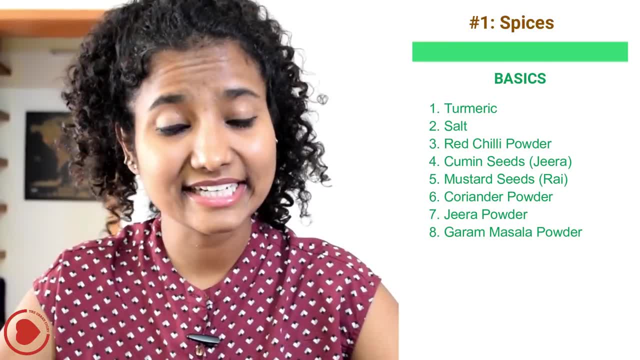 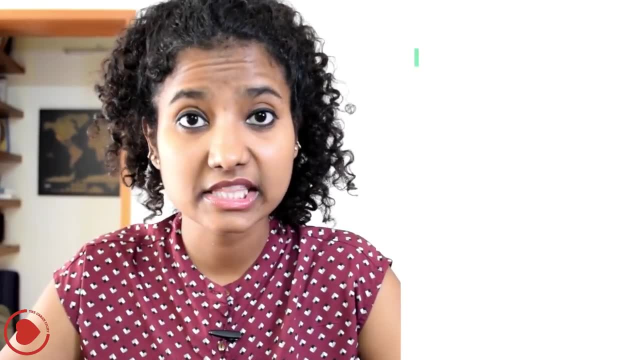 That's all the spices you will ever need. The final category is hara masala, coriander, kariya pak and hari mirch. I strongly suggest that you buy them fresh every week. Next thing that you need in your kitchen are called staple items. These are the things that you must. 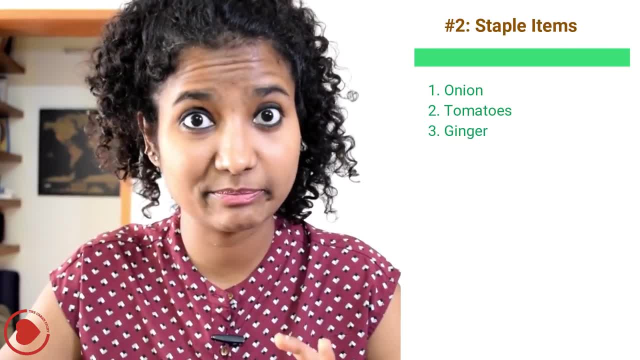 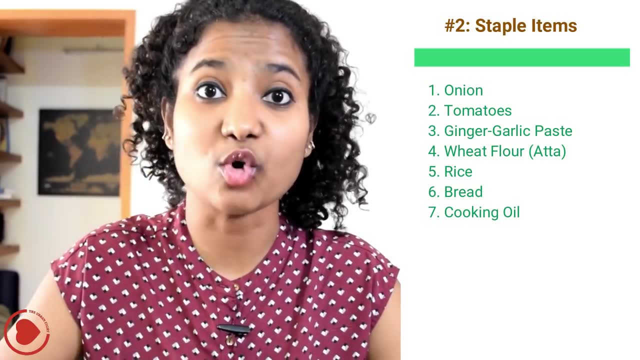 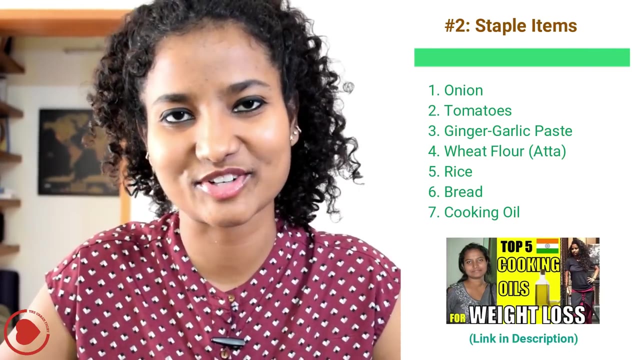 have in your kitchen: Onions, tomatoes, ginger, garlic paste, atta rice bread and oil. In case you want to know which oil is best for weight loss and for health, then check out this video. I've left the link in the description. 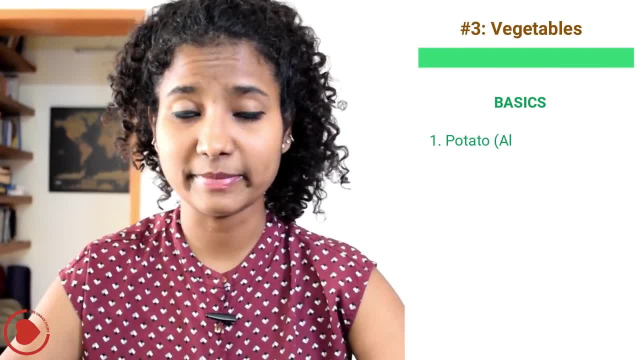 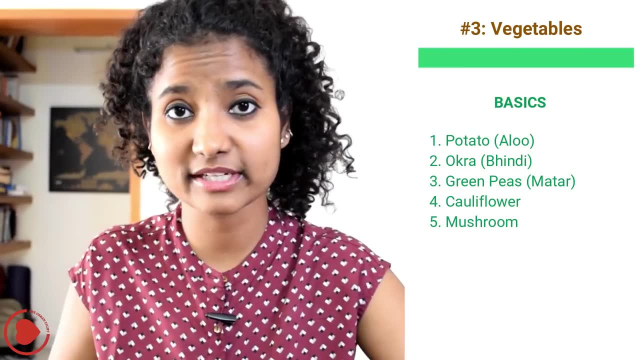 The next are vegetables. The basic veggies are aloo, bhindi, mutter, cauliflower and mushrooms. You can make like a gazillion permutations and combinations using just these. First, you need to prepare the vegetables. You can make like a gazillion permutations and combinations using just these. 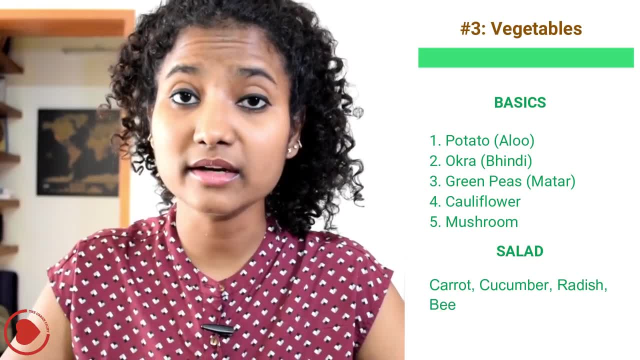 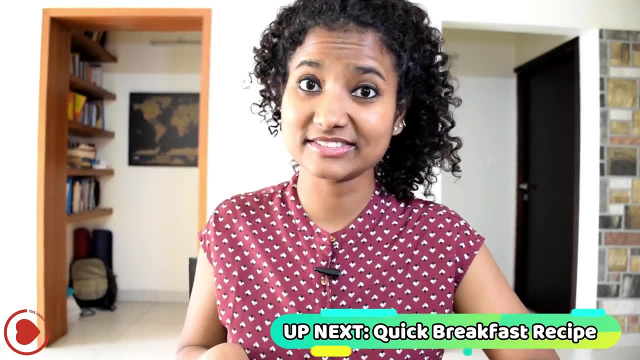 For salad. get some carrot, cucumber, mooli or beetroot- Just get one of these every week- And also some lemon. I know I missed a lot of vegetables, especially the ones that are local to your state, But it is your job to find out what they are. 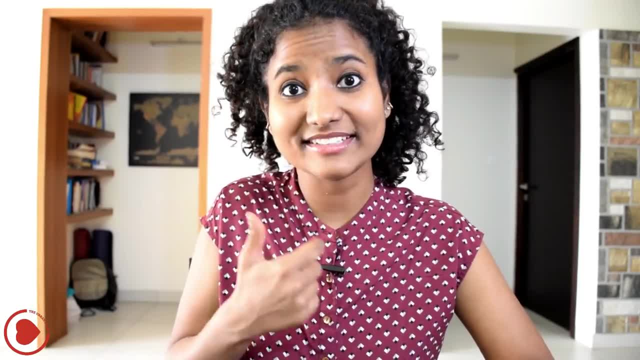 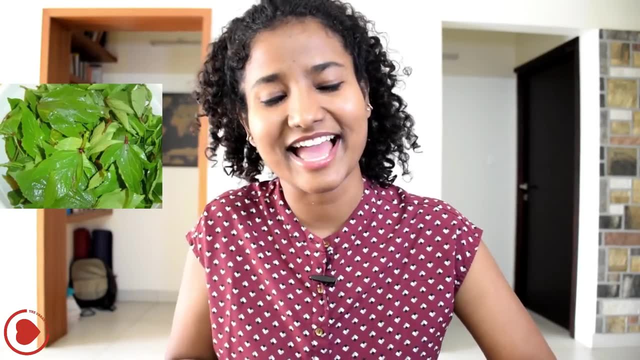 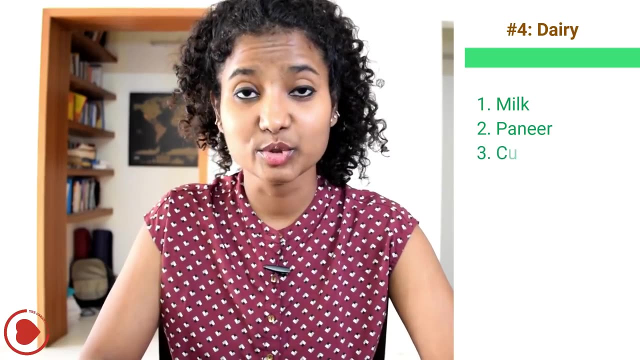 and then tell me which state you're from and what is the vegetable that is local to you. For example, I am from Hyderabad and we have ambade ki bhaji And I love ambade ki bhaji. Anyway, next is milk products, Milk paneer and curd. You will use these extensively if you graduate to making. 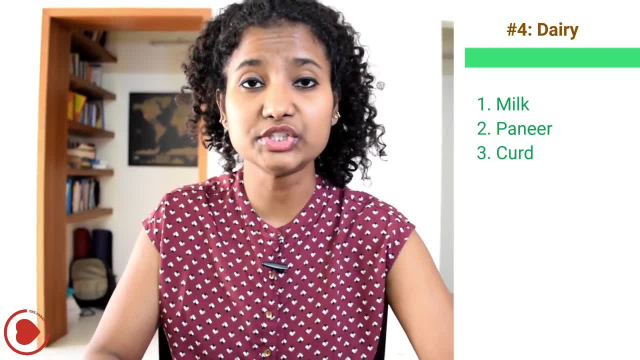 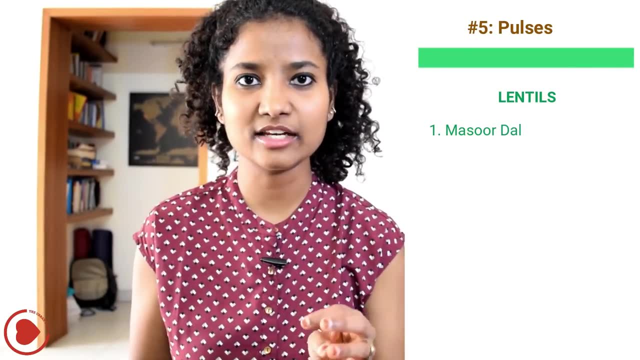 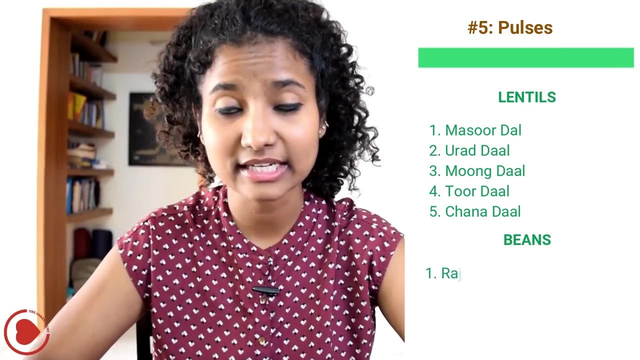 shahi items, Or even chicken, because they make the dish YUM, Especially curd. The fifth category is pulses In dalt. we have masoor dal, urad dal, moong dal, toor dal and chana dal. Chana dal is like my absolute favorite dal, And then come the beans Rajma. 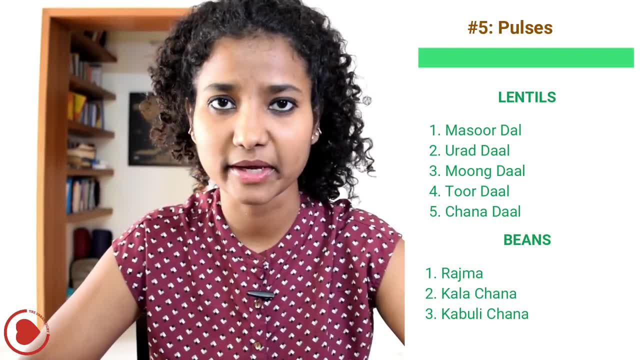 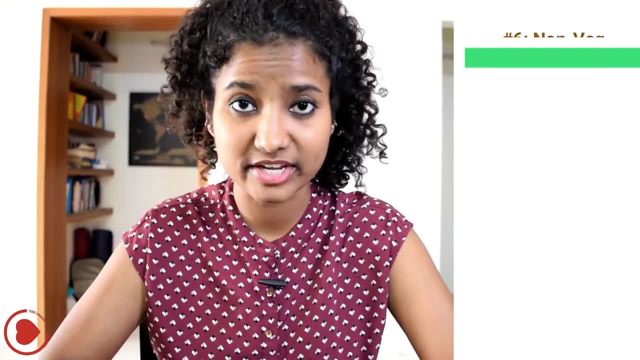 kala chana and kabuli chana, which is used to make chole. by the way, You don't have to buy all of them. For starters, just buy one dal and one bean. And the final category is non-veg. If you're non-vegetarian, 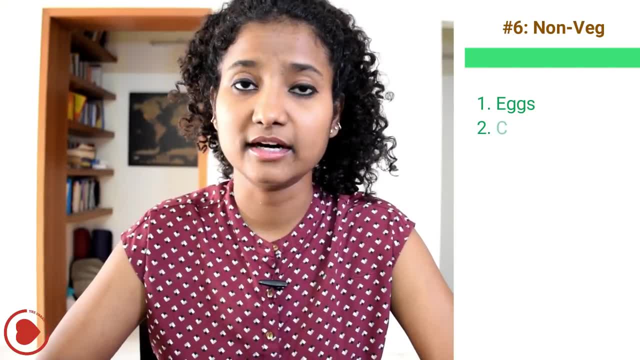 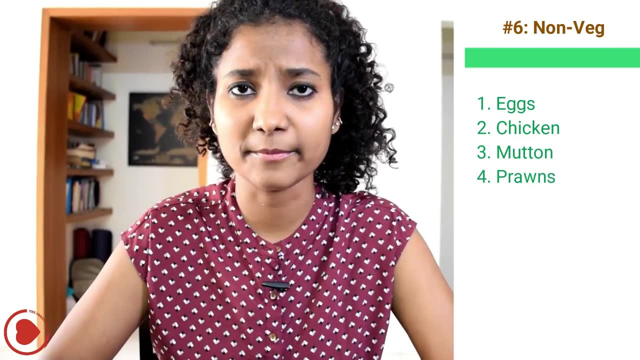 then A eggs is like the go-to breakfast option ever. B chicken is the easiest thing to cook if you marinate it and time it right. Then you also have mutton prawns, fish. It basically depends on what you like to eat, And that's all the things you need in your pantry If you want me to make a separate. 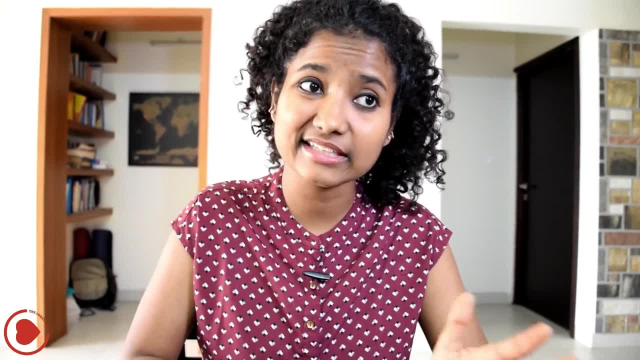 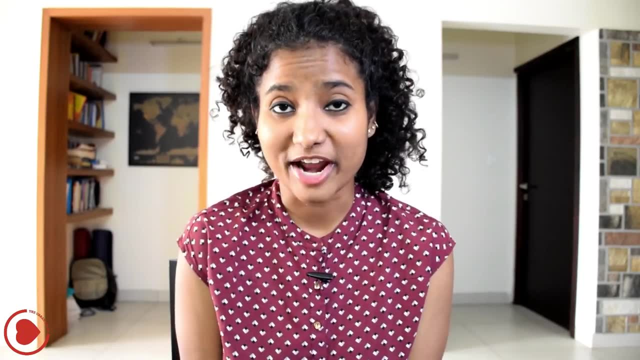 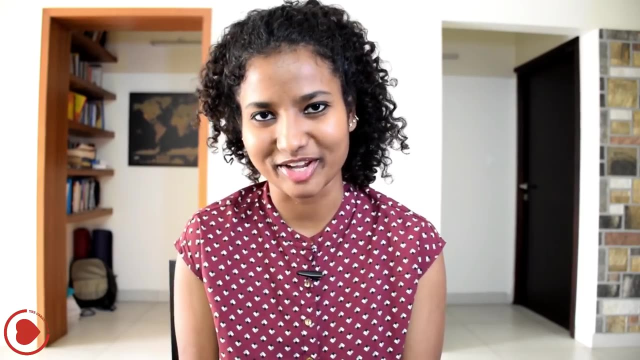 video a part two, including the utensils and the kitchenware you need in your kitchen. then comment and let me know. Day two breakfast, Now that my pantry's tagged on day two. I started simple by making an easy paneer sandwich for breakfast. First, grill two bread pieces. You can even use a normal pan. 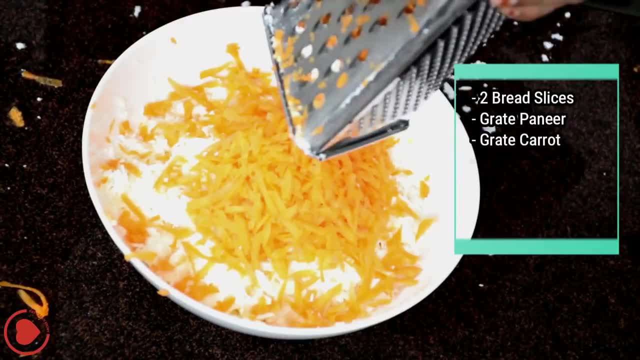 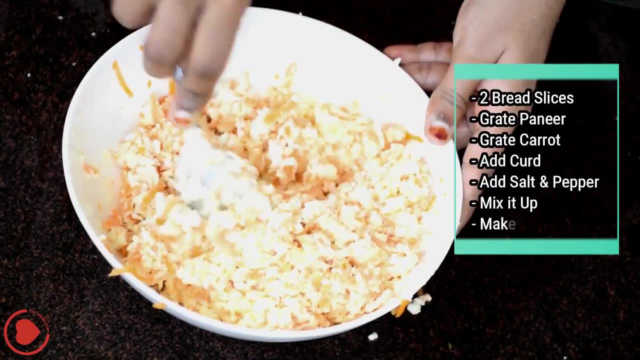 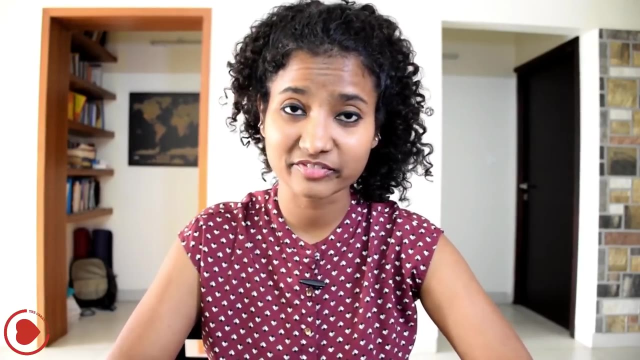 Take a bowl grate paneer, grate some carrot, add a little curd salt pepper, mix it up and my stuffing is ready. I just place it between two pieces of bread and that's it. That's my breakfast. After that lip-smacking breakfast, I slowly ease into day number three. 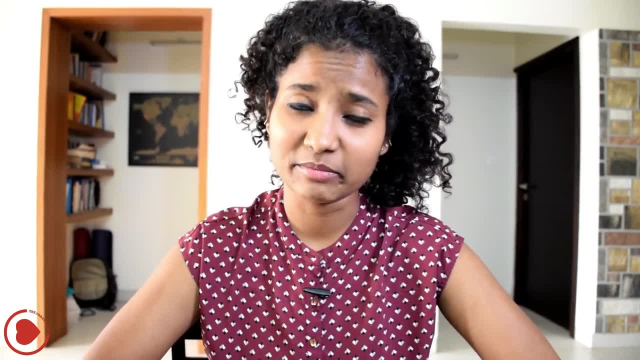 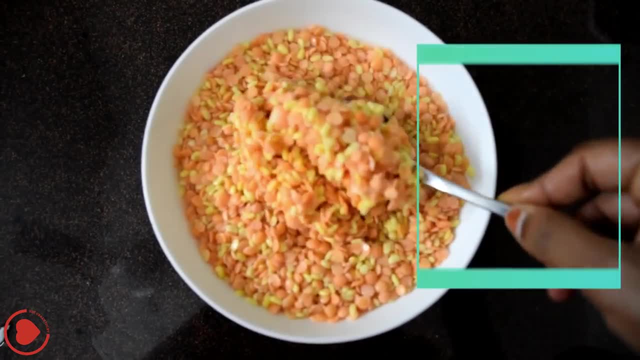 On the third day, I made dal, and it is the easiest thing to make, because now that you have your masalas, it's just a matter of adding them one after the other, Wash and soak the dal for 30 minutes. I usually mix two dals together, masoor and moong, this time. 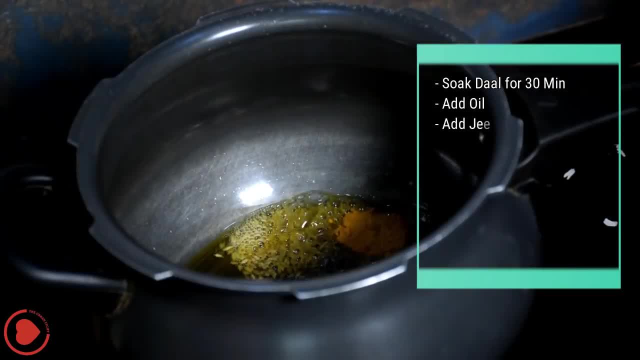 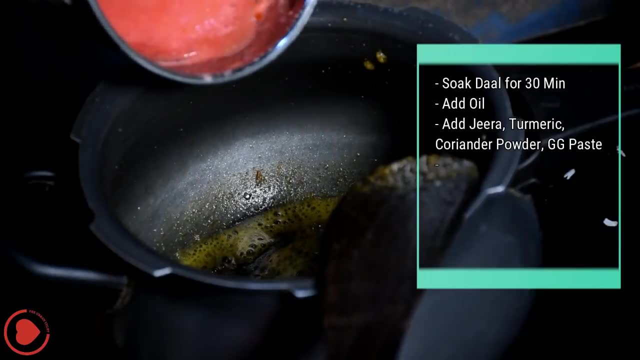 In a cooker. add two spoons of filtered oil. Add jeera, turmeric, coriander powder, ginger-garlic paste and fry them a little. Now add a tomato. You can chop the tomato or make a paste. I like to make a paste. 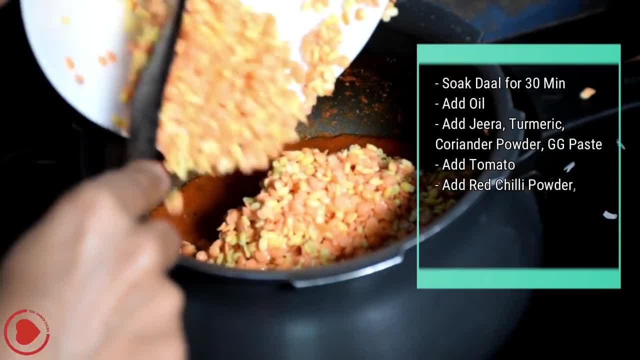 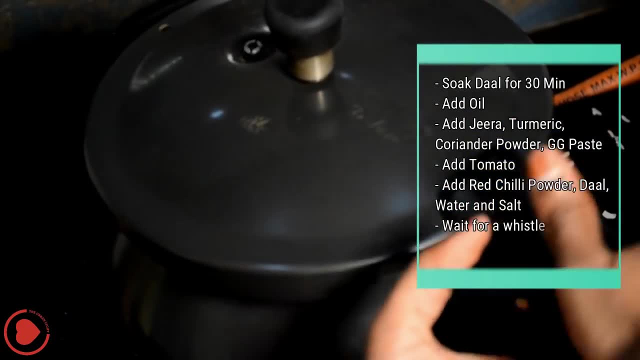 Add some red chilli powder. Finally, add the soaked dal and fry for a minute. Add some water salt and close the cooker lid And wait for one whistle. In the end, add some coriander, if you want. 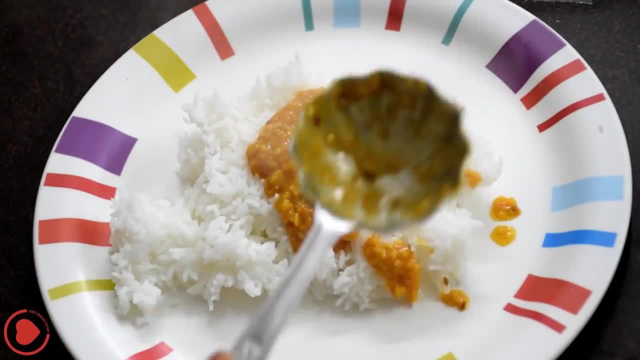 and you're done. Make some rice roast, some papad and your perfect home-cooked meal is ready. Now let's advance from dal to dal to dhal. To make dal, you need to mix urad dal and urad dhal. 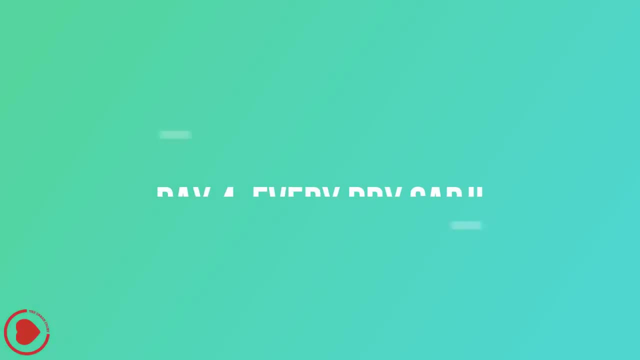 You can add urad dhal in a bowl too, To make dal. I'm adding urad dal in a bowl and I'm adding urad dhal in a bowl. Now let's advance from daal to vegetables. Day number 4.. 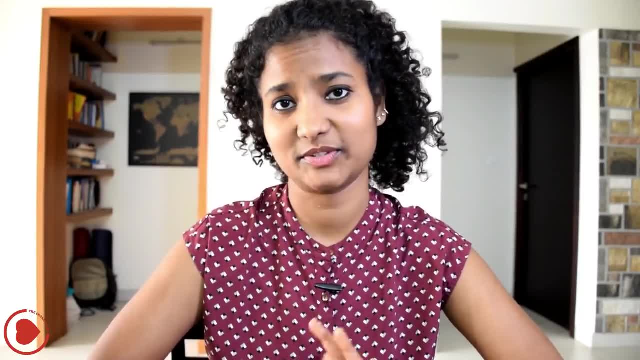 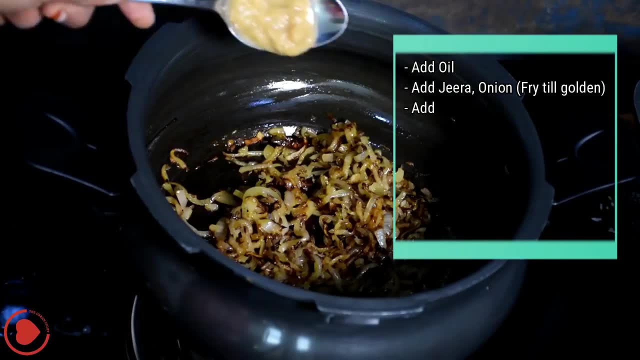 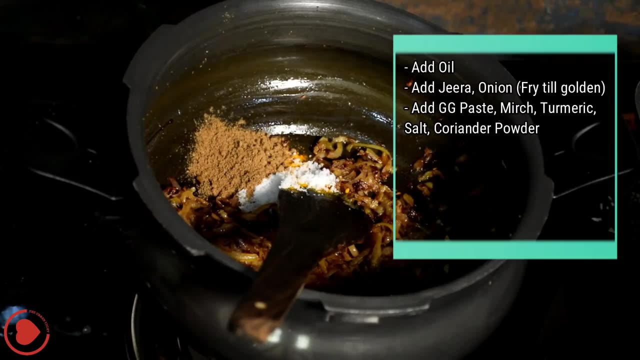 The procedure to cook any dry Indian curry is this: Add oil, jeera onion and fry till the onion turns golden brown. Now add agar, glesan, harimirch, haldi salt, dhaniya powder and fry these masalas for a few seconds. 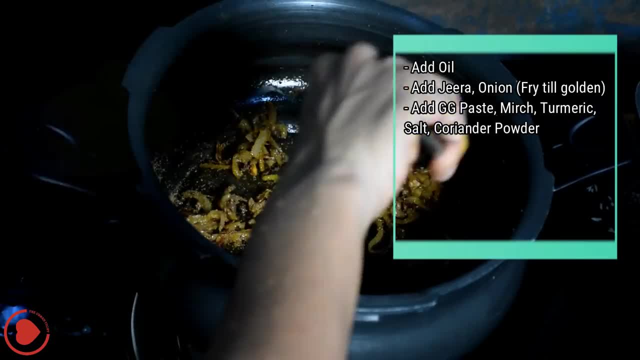 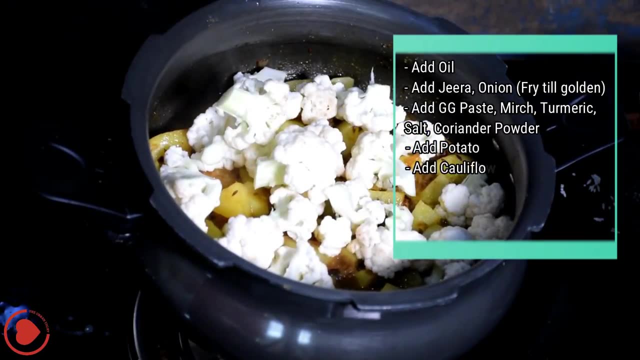 Now to this mixture you can add any vegetable that you want: Aloo, gobi, mushroom, matar. I am making aloo, gobi, so I'll first add aloo and then gobi, Close the lid and cook it on low flame. Add a little garam masala on top, Mix it well and we are done. Thank god for whoever invented this procedure. You can cook any Indian dish. The different vegetables used and the quantity of spices is the reason why every dish tastes different. 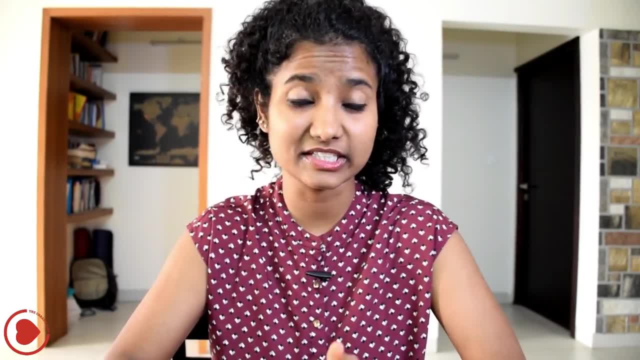 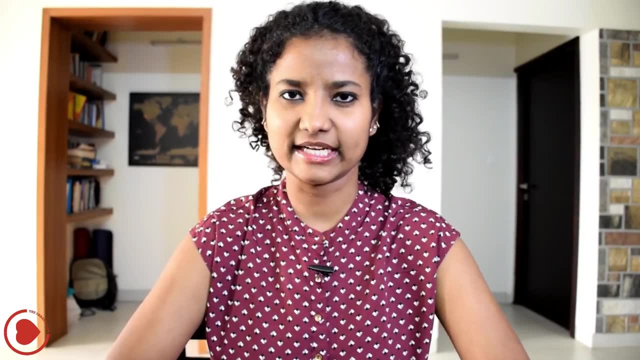 Day number 5.. Now, after you have graduated from the regular dry sabji, it is time to up your game. I call it the YouTube cooking. Suppose I want to cook something complicated like palak paneer. I'll search for that dish on YouTube. 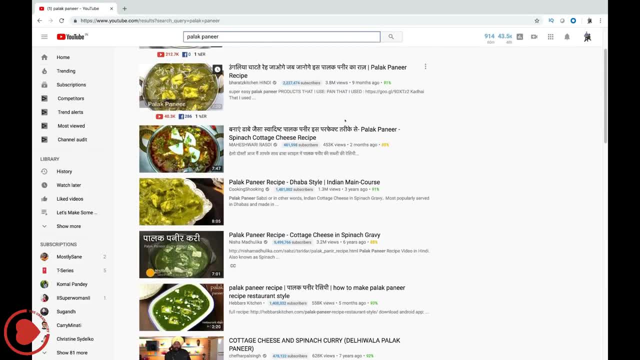 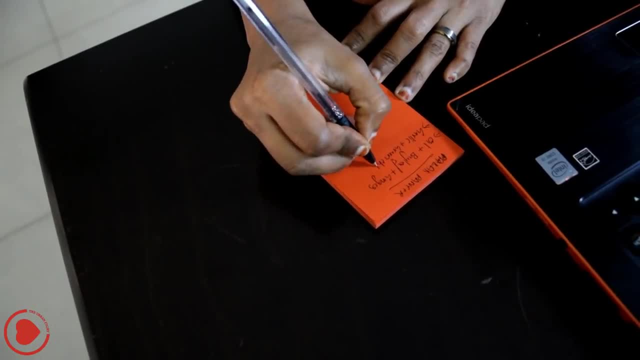 Watch 4-5 videos. My aim is to find a recipe that is neither too complicated nor too simple. This is the one I like so far. I write down the recipe on a post-it, Hang it on my fridge next to the other recipes I've collected over time. 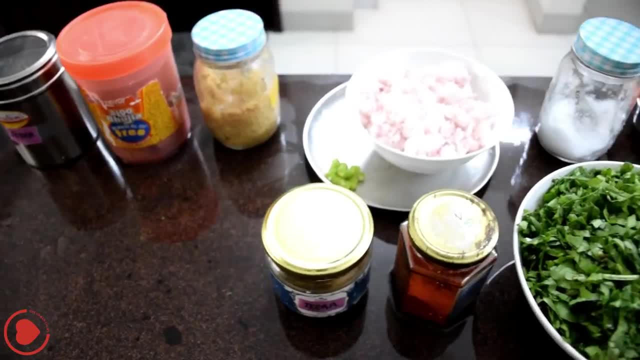 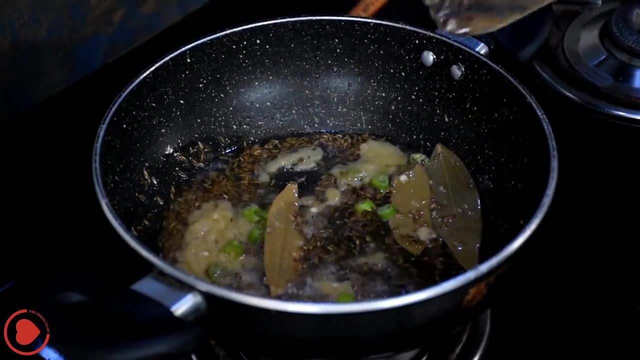 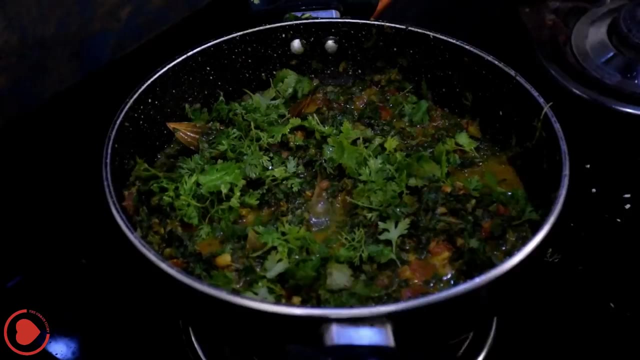 Now it's all about following the instructions to the dot. I first get all the ingredients ready and lined up in order, And then the cooking begins. I'm not going to lie, It takes a little bit more effort than usual, So I reserve this only for Sundays. 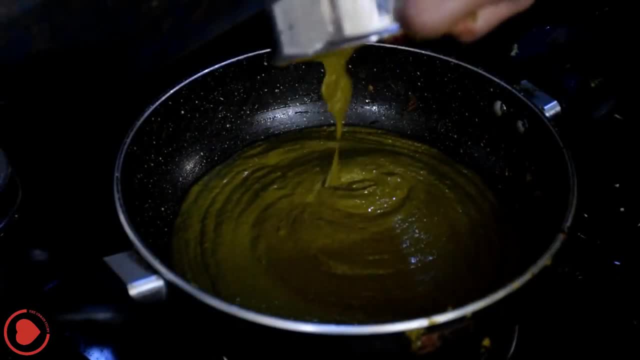 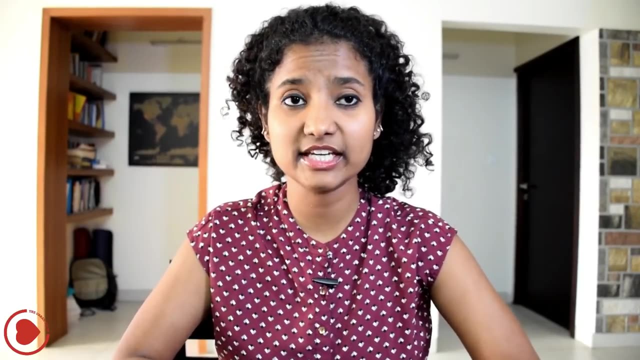 But it's all worth the effort Because in the end the dish turns out pretty great actually, And for that I cannot thank the cook. I can't thank the cooking channels enough, Especially Cook with Lubna Kabita's Kitchen, Bong Eats and a blog called Maika. 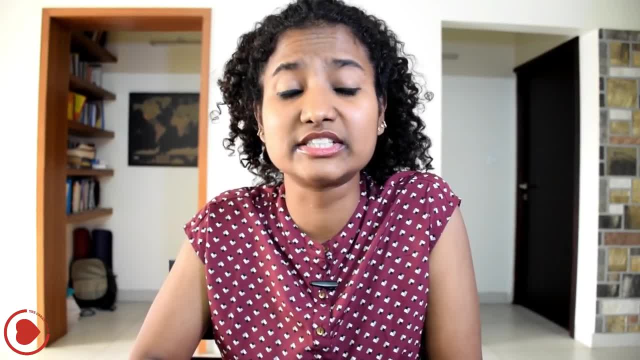 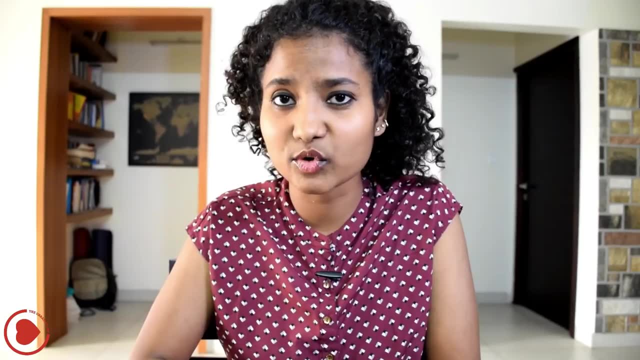 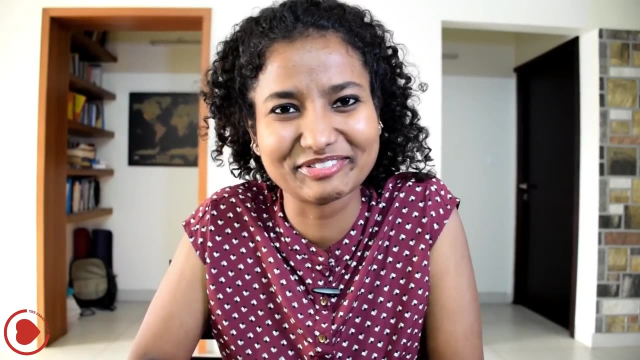 But the lady that I absolutely adore is Nisha Madhuleka. She literally taught me 70% of the cooking that I know, So if you want to learn how to cook, go to her channel and subscribe right away. And while you're there, can you please request her to do a collab with me? 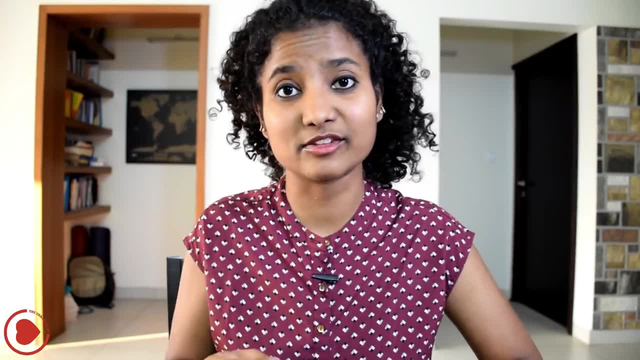 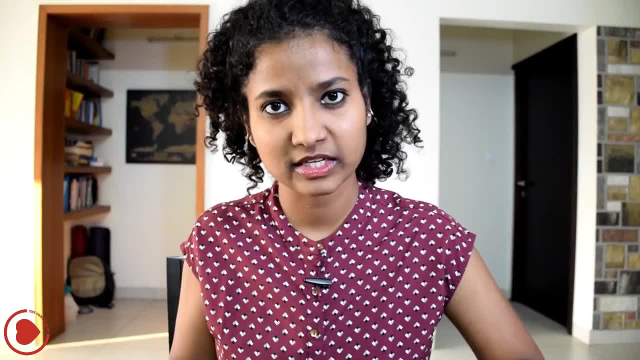 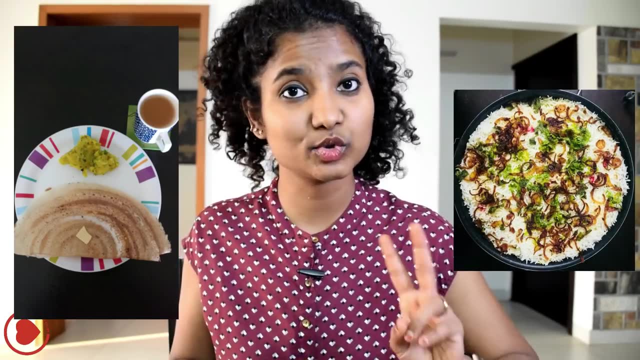 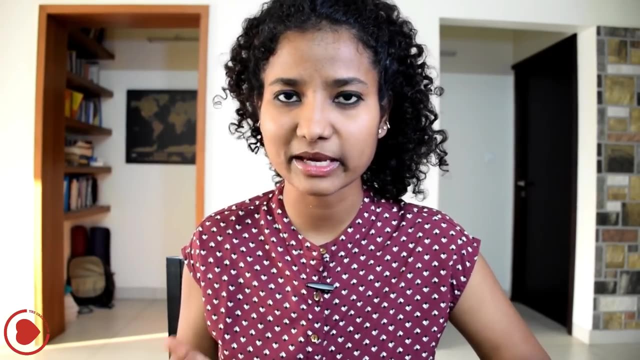 know is cook is your family recipe. My mother taught me how to make dosas And my mommy taught me how to make biryani, And these are the 2 dishes that I make the best. In fact, I think half of my friends are friends with me because I make biryani on Eid. 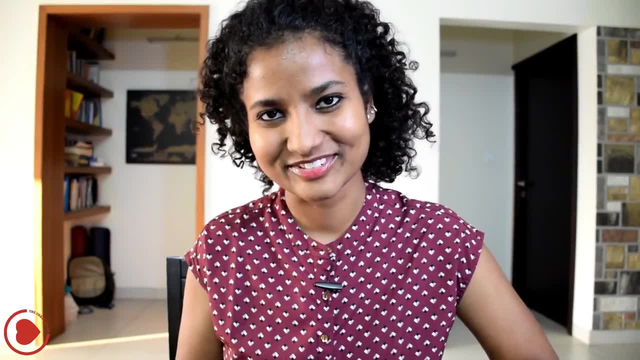 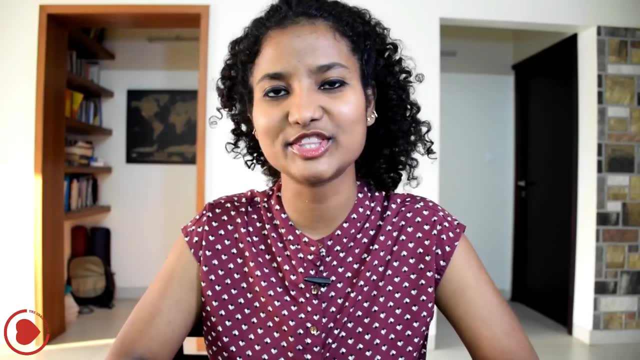 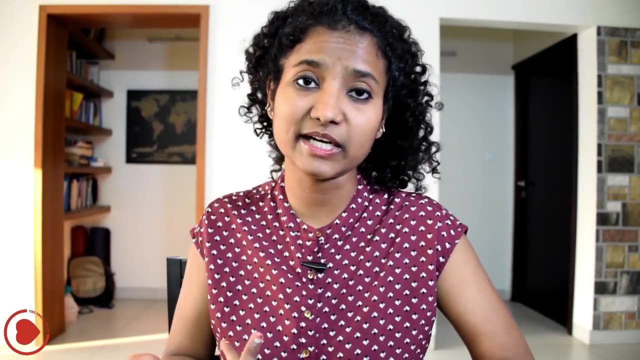 So call in and tell me what is your favorite family dish. And while you do that, make sure you subscribe and hit that bell icon, because I make health and wealth videos every Thursday, Only on Eid, for you. and finally, here's the bonus tip: as soon as you enter the kitchen, do not expect to turn. 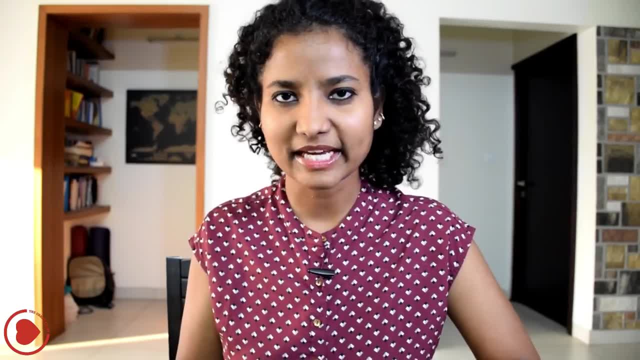 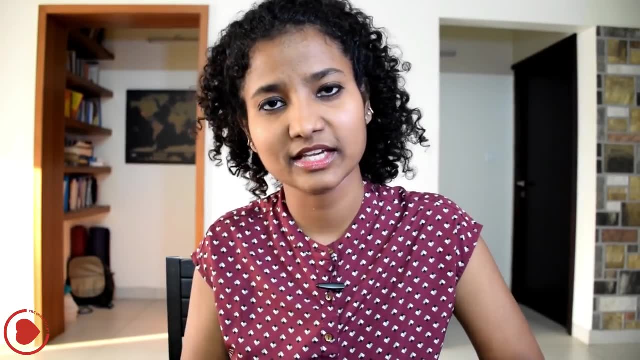 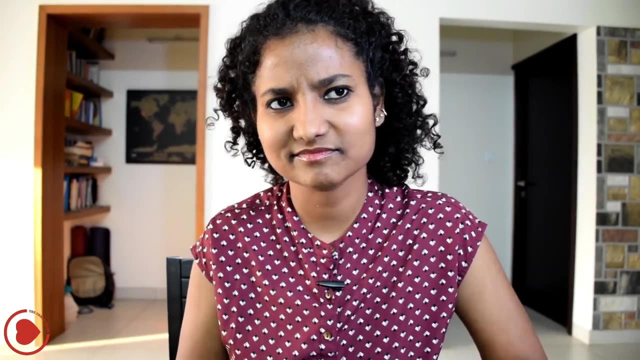 into tarla dalal or sanjeev kapoor. sometimes you will put less salt, sometimes you will put more on some days you will burn the whole damn thing, but you did not give up. after you fell from the bicycle for the first time, did you then? why quit cooking? it takes a week or two to learn how to.